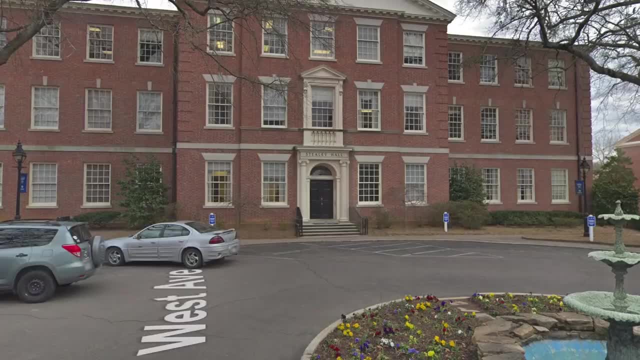 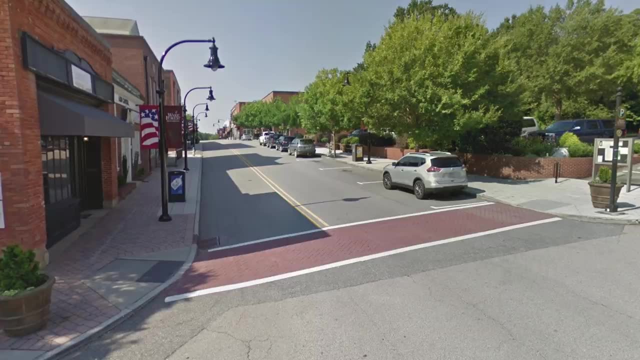 42,000 people here. This was once home to Wake Forest University, but they moved to Winston-Salem. It's a small, close-knit community. It's perfect for families and people who want small-town community life. The downtown's awesome and really quiet. There's no homeless people here. that's for sure. There's a lot to do in Wake Forest. There's museums and breweries, but it's kind of a small-town lifestyle. It's different than Raleigh and it's only 30 minutes away, so you can go to Raleigh if you want fun Now, like a lot of other places on this list. 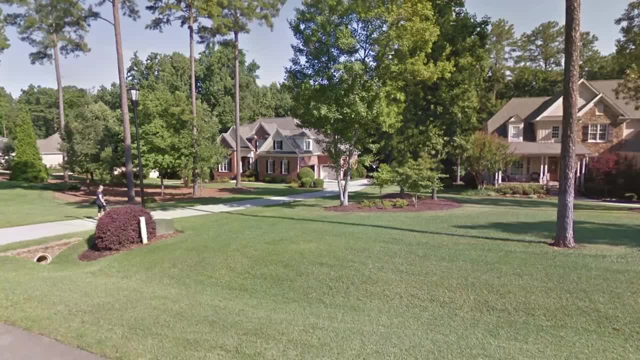 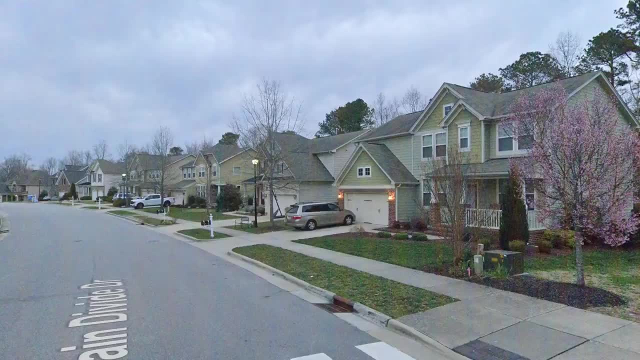 the median salary for people living here is going to be pretty high, about 92k a year for the family, and homes are about 300k. That's right. Wake Forest is actually more expensive than Raleigh, but you get what you pay for. It's quiet and safe, the schools are good and, like a third of the 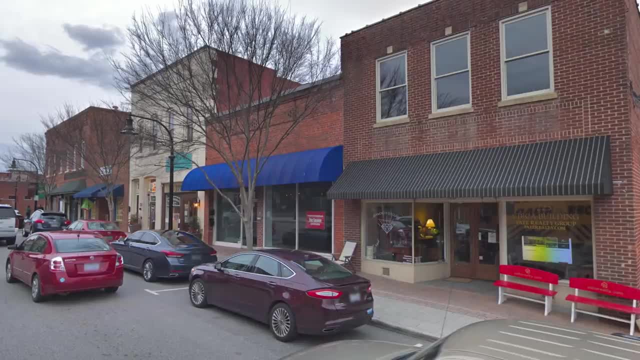 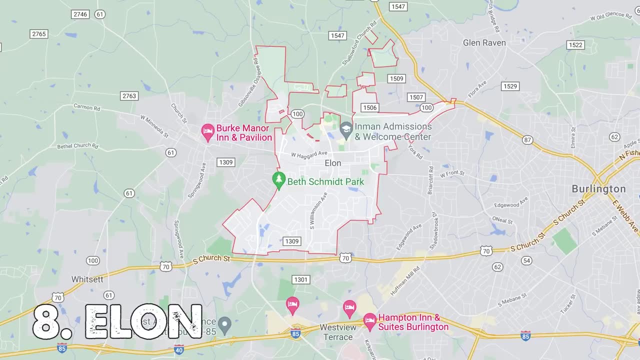 population has a bachelor's degree, And it's not just for families here either. Wake Forest was also called one of the best places to retire. At number eight is Elon, Outside of the Raleigh area. it's way out by Greensboro in Alamance County. There's 12,000 people here, but it's growing fast. 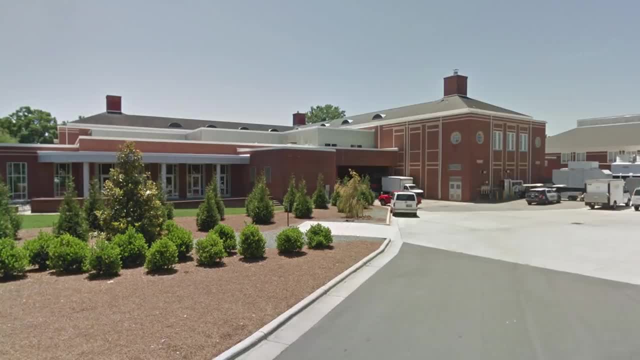 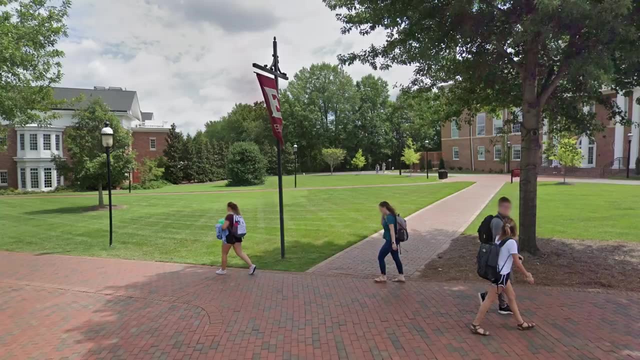 It's home to Elon University and because it has a lot of college students, it's going to have a young population. The average age here is 22,. but Elon's not like a normal college town. It's actually quiet and safe. In fact, it was called the second safest city in the state, Just about. 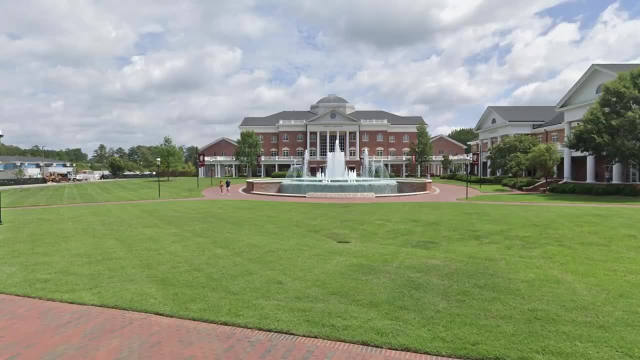 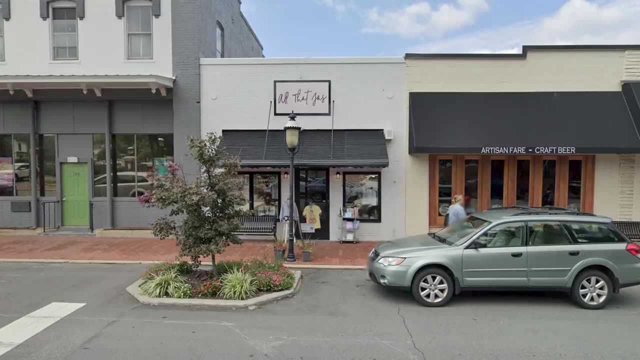 everybody in town has a good job too. People who live here say Elon's a beautiful town with a heart of gold. They say people are always friendly, no matter if you're a friend or a stranger. Maybe everyone's in a good mood because they don't have to sit and 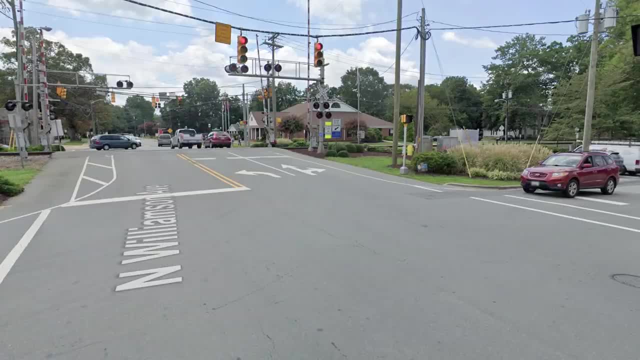 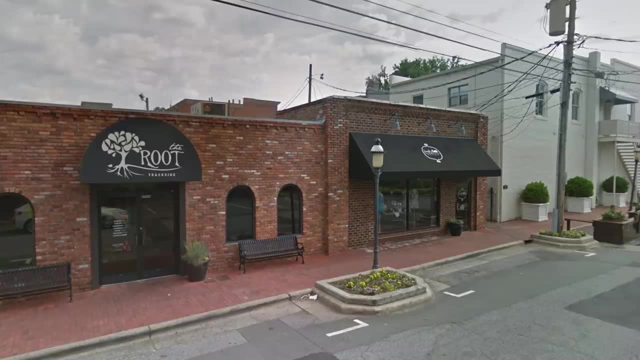 traffic. I mean people who live in Elon have one of the shortest commutes in the state. The only drawback is you'd probably have to drive to Greensboro or Winston-Salem for work, and those places are not very charming For being such a small town. there's actually a lot to do. 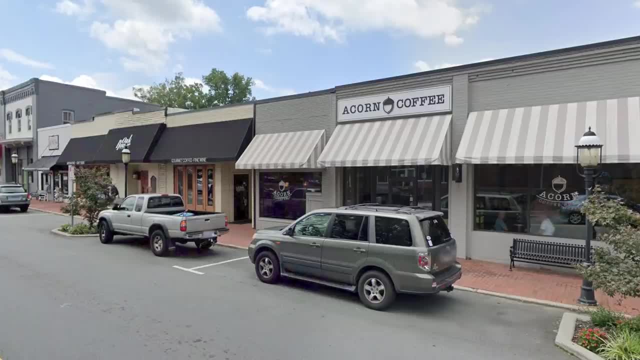 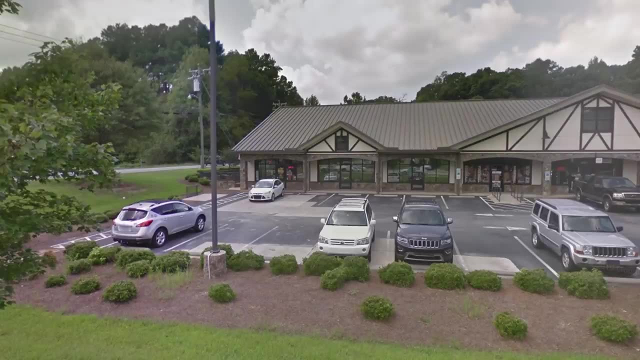 in Elon There's cute little restaurants and coffee shops and places to shop. If you're looking for live music, you can find a lot of locals at the Fat Brog on the weekends. And no, the Fat Brog did not pay me to say that Now the seventh best place to live is going to be way out in. 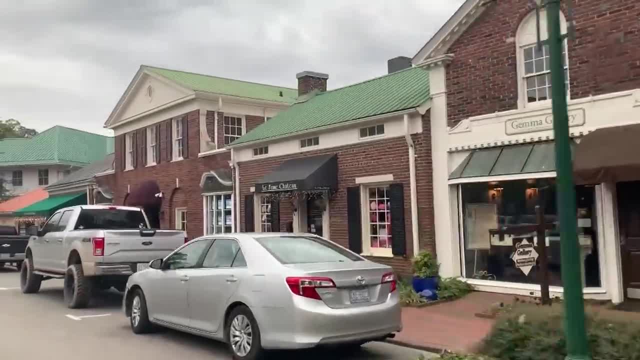 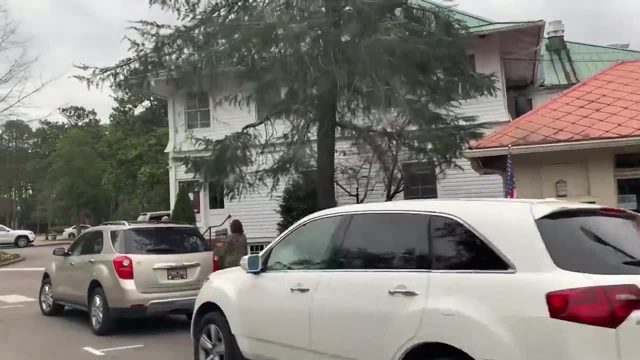 Pinehurst down in the Sandhills region. It's about an hour southwest of Raleigh. There's not a lot around here, but Pinehurst itself is awesome. There's only about 16,000 people here and it kind of feels exclusive. The location's great. I mean, you're two hours from the beach. 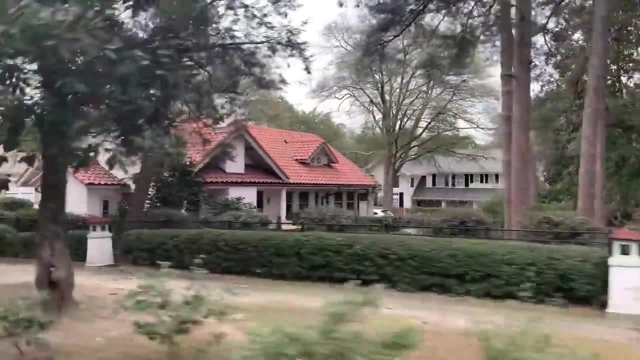 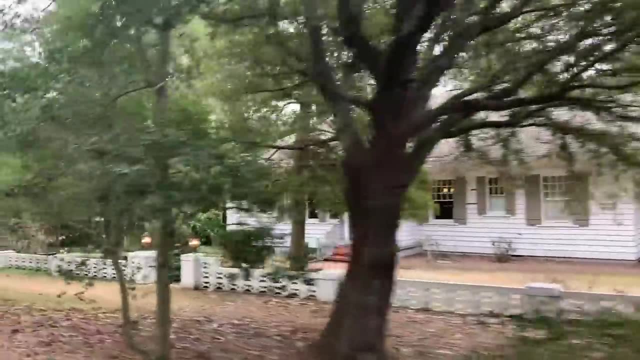 and two hours from the mountains, but you're kind of isolated way out in no man's land. Of course, Pinehurst is kind of a golfing community. The village is home to some of the most famous golf courses in America, including Pinehurst Resort, which has hosted a bunch of 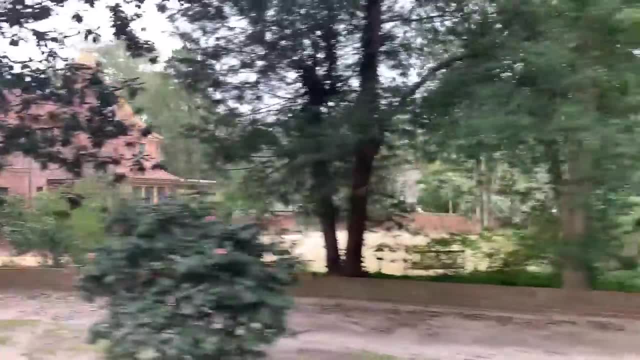 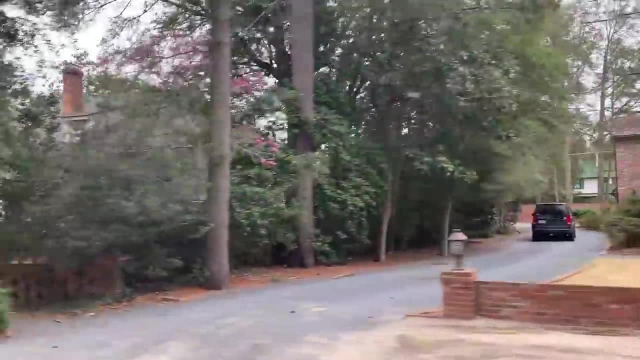 events, including three US Opens. Pretty much everybody here is retired or has a good, high-income job. A lot of people work from home. Now, if you don't have a job outside of health care and hospitality, there's not a lot of options. You better bring work with you And believe it, or 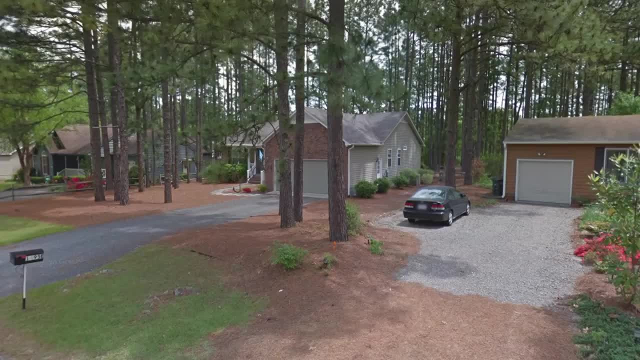 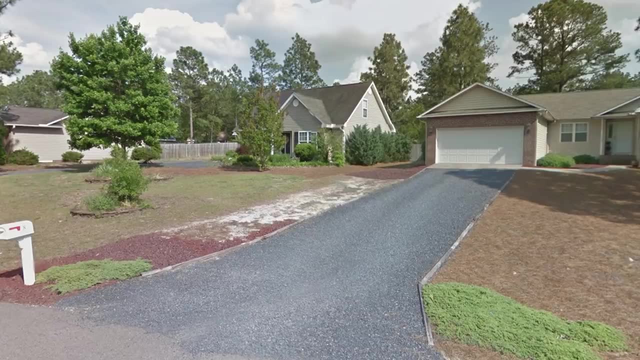 not. there's actually areas in Pinehurst that are still sort of affordable. I mean, the median home price here is $293K and property taxes aren't that bad either. Overall, Pinehurst is easy to get around. It's super family-friendly and there's activities for kids and there's a 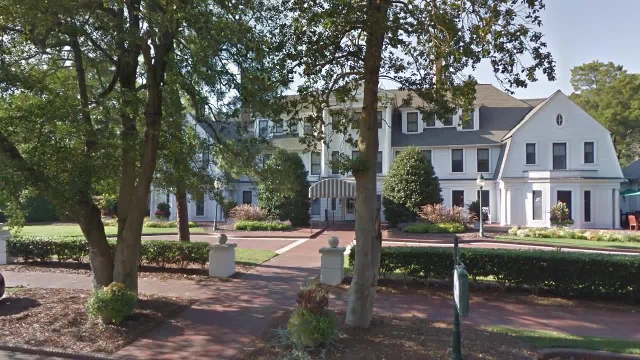 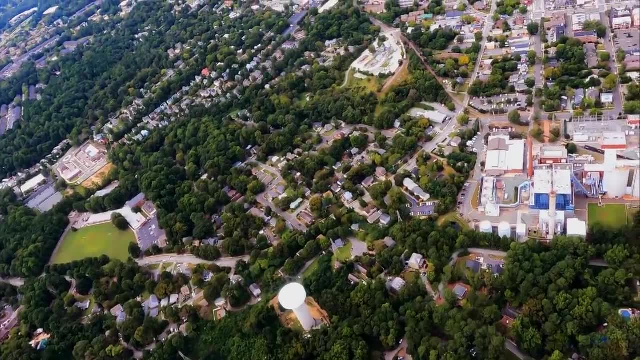 vibrant culture, but it's probably more of an older crowd At number six, Chapel Hill. Hey, I used to live in Chapel Hill. I know a lot about Chapel Hill. It's about 30 minutes from Raleigh and 15 minutes from Durham, which sucks, But again, it's part of the Triangle area and the 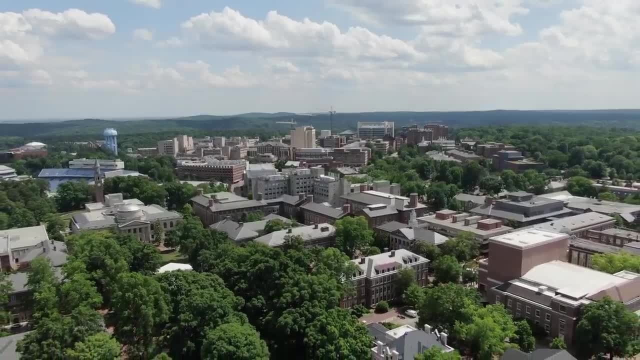 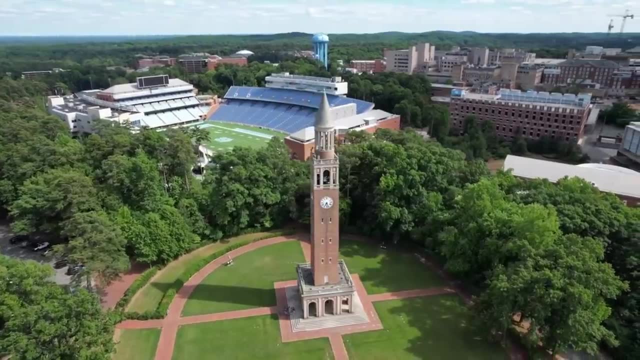 Raleigh Metro area. There's 60,000 people in Chapel Hill and of course, it's home to the nation's first public university, the University of North Carolina, which has the best sports in the country. So because of that, there's a lot of young people in town. 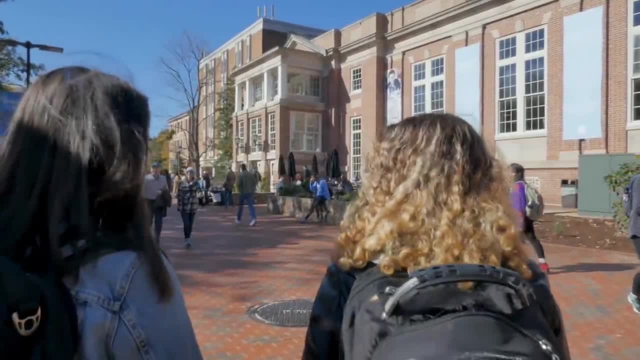 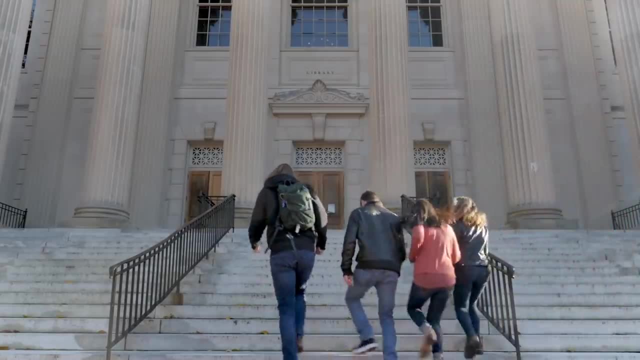 However, it's also kind of a retirement community, or it seems like it. It feels like if you're in your 30s or 40s, there's not going to be a lot of people your age- Everyone's either 25 or 65 in. Chapel Hill And it's really expensive. I mean, Orange County has like the highest taxes in the state and the home prices are the fifth most expensive in the state too, at like $400K. But you get what you pay for. It's really really safe. The schools are the best in the state. 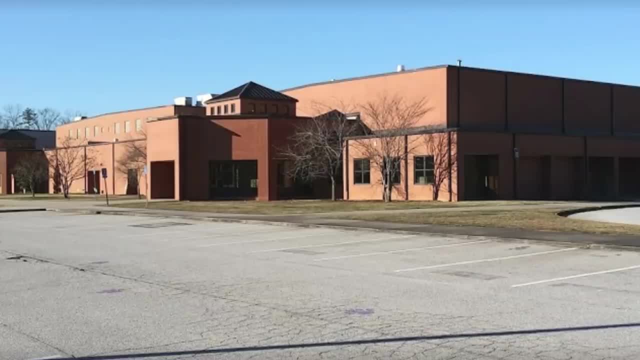 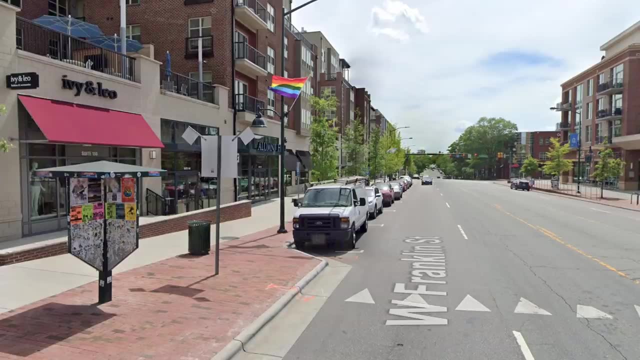 and three and four people here have a lot of money So it's really really safe. A college degree- So a lot of people are smart. You can't go wrong with Chapel Hill if you can afford it For fun. it's going to be mostly wandering around on Franklin Street down near. 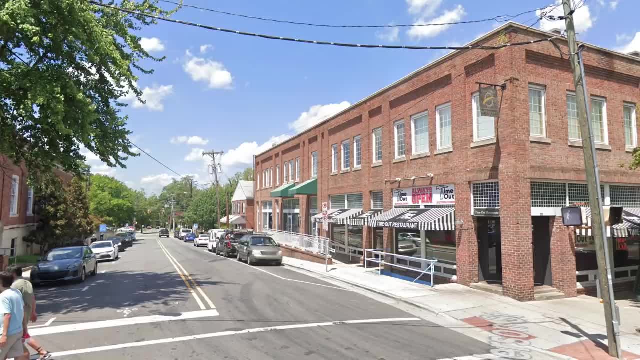 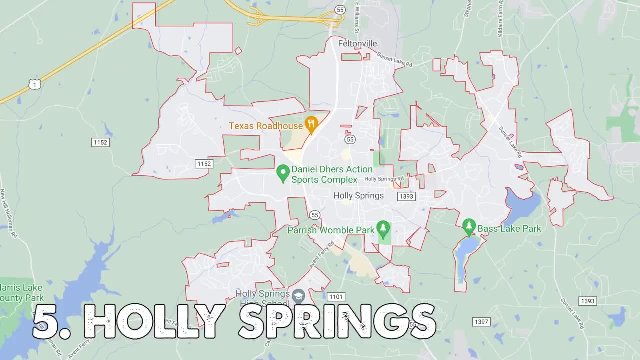 UNC's campus. There's a bunch of shops and places to eat. There's all sorts of stuff going on on campus every single day. Chapel Hill is a great place to live Now. Holly Springs is about 20 minutes from Chapel Hill. It's also in the Triangle region. There's 35,000 people here. 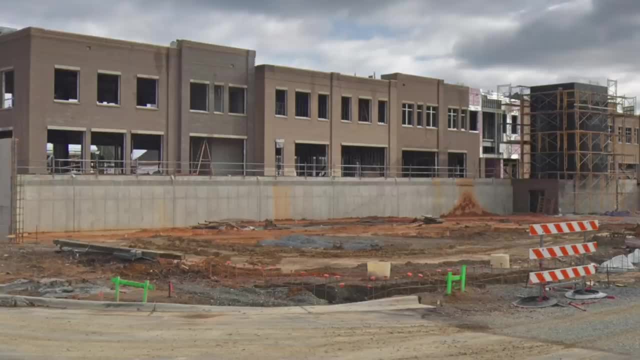 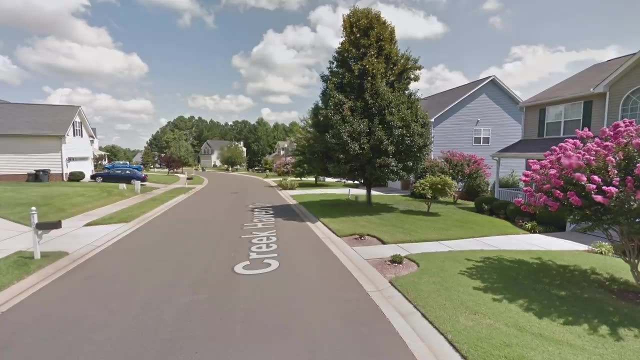 but this place has almost doubled in the last five years. They can't build homes fast enough here. If you want to live somewhere that's really safe in the middle of the Triangle area, Holly Springs is a good choice. It was also voted as the best place to raise a family in the whole. state Again. the schools are great, It's super safe, It's really pretty and it's really not even that expensive, relatively speaking for where you're from, And even though it's grown fast here, Holly Springs still kind of feels like a small town. I mean there's plenty to do here. 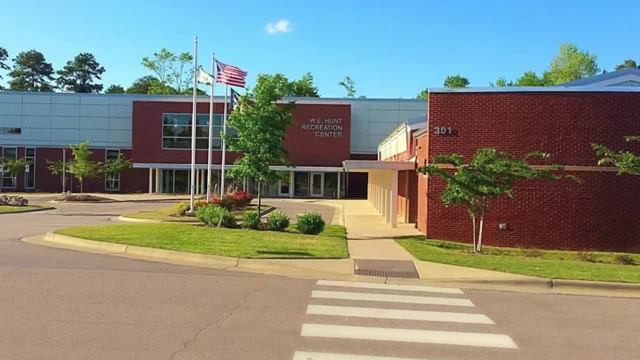 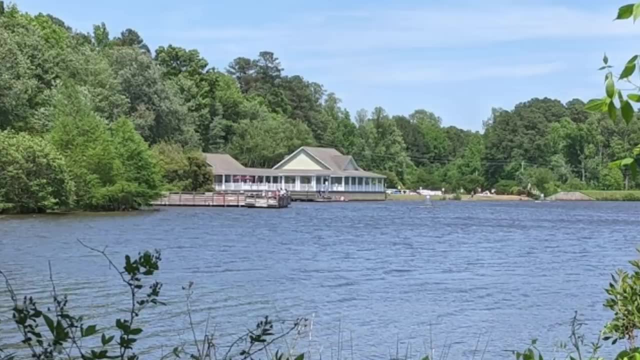 The city just invested a hundred million bucks for public infrastructure, for parks and recreation and shopping and dining. They have free concerts in the summer and they have holiday festivals in the winter. Now, right next door is Morrisville. Are we seeing a pattern here? Just about all the 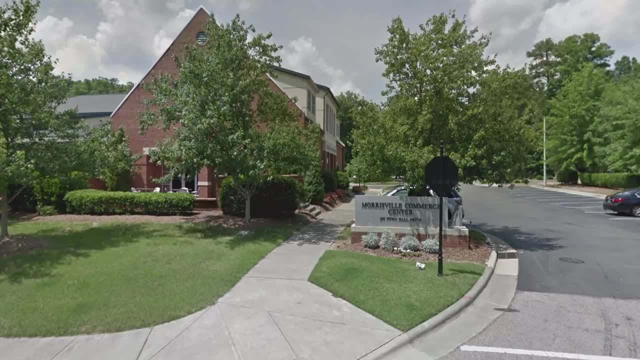 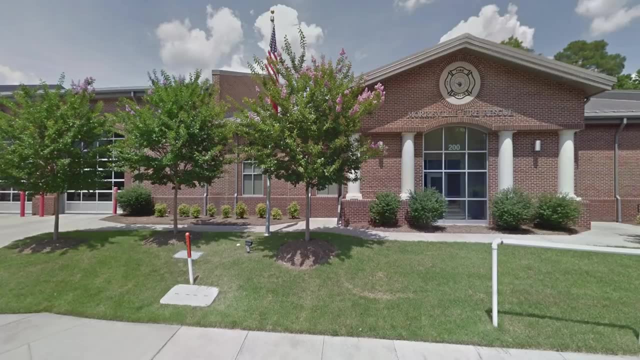 best places to live are going to be in the Raleigh metro area. Morrisville has about 25,000 people here and it's also growing really fast And, just like the other places on this list, it's going to be super family-friendly: Half of the households have kids and the public schools are in the top. 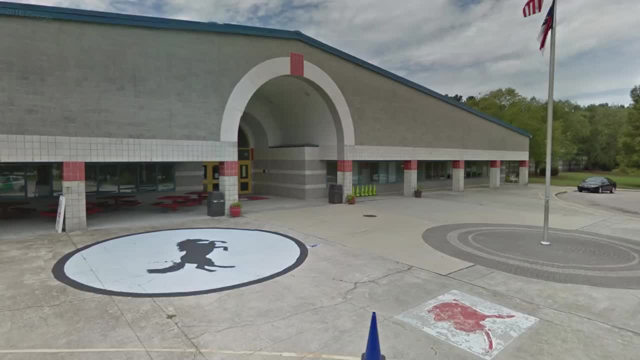 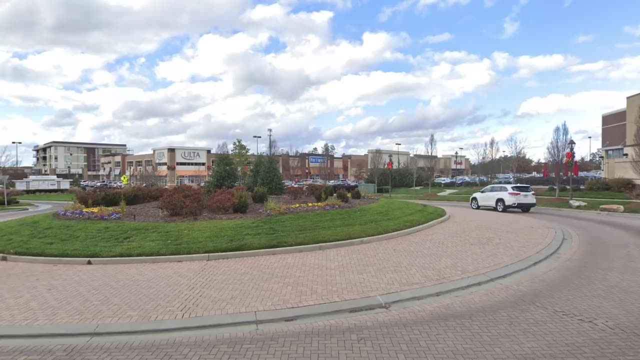 five percent in the state. They also have the 10th lowest high school dropout rate in the state too. Two-thirds of Morrisville residents have a bachelor's degree. That's more than double the state average people, And you hardly ever hear about crime here. They have the. 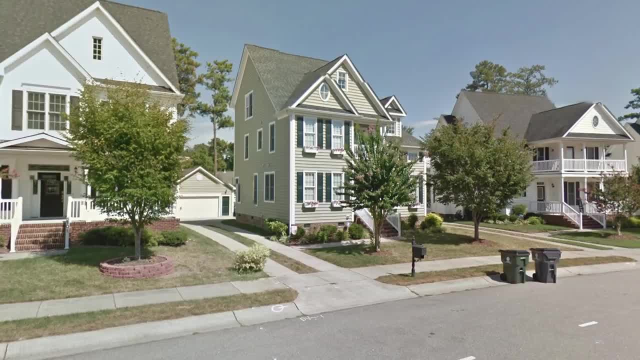 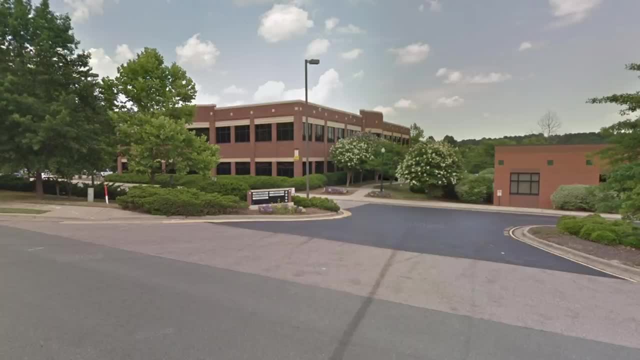 third lowest violent crime rate in the state and there's great tech jobs all over the place. Like you could drive 10 minutes to work. There's that many good tech jobs in Morrisville, and health care jobs too. Now Morrisville is going to be a little bit more expensive than some of the other. areas in the triangle. It's about 350k for a home on average, but the good ones are going to be closer to 400k. Right next door is Apex. Now they call this place the peak of good living. The schools are. 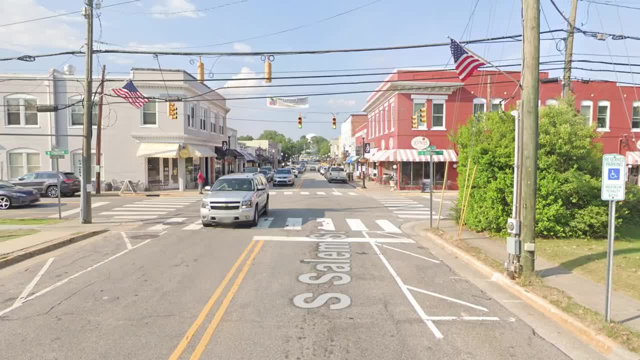 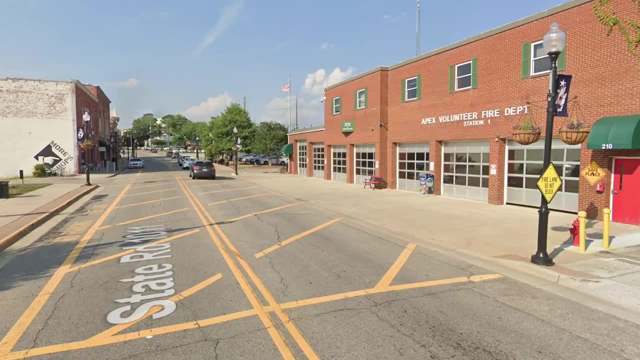 great. There's a charming downtown and lots of people are involved here. If you don't have a job in Apex, it's because you don't want a job. Everybody in Apex has a good career and earns pretty good money. It's going to be a little bit cheaper to live here than next door, but that's. 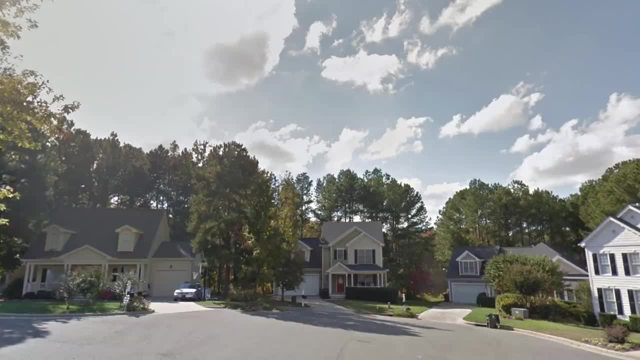 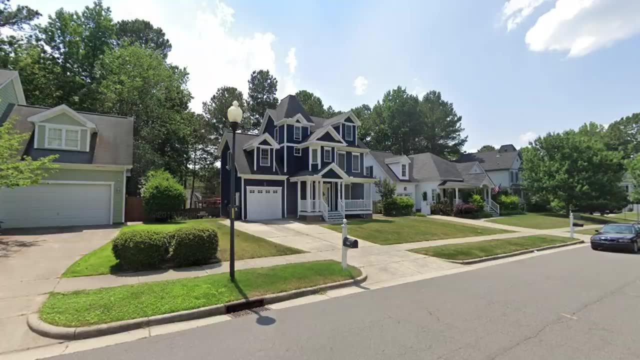 because it's more spread out and doesn't really have a center of a downtown. in Apex, Homes are about 330k but they're going up all the time. people I know there's people in California that are like: wait, I can pay half as much for a house and have twice as much safety. Yes, you can. 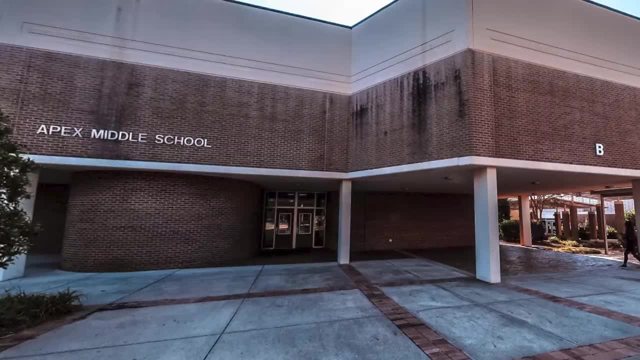 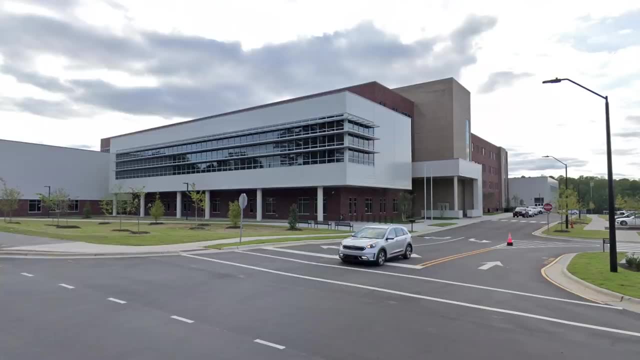 Like Morrisville, Apex has one of the best public school systems in the state. Only 2% of adults never finished high school here and like 40% of people went to college. There's going to be parks here, outdoor activities, farmers, markets and festivals, just like everywhere else. we've talked. 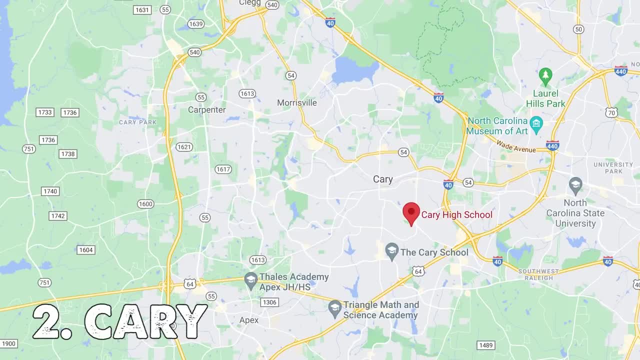 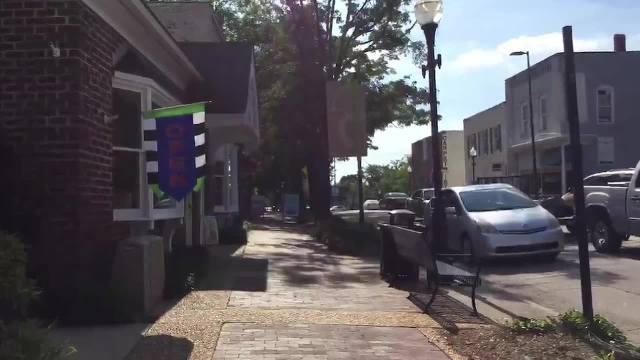 about too. And right next Next door is Cary. Now, this is the closest suburb to downtown Raleigh. Now talk about family-friendly. This whole place is filled with young families with a bunch of kids. If your kids are into sports, there's endless sporting leagues and things going on on the 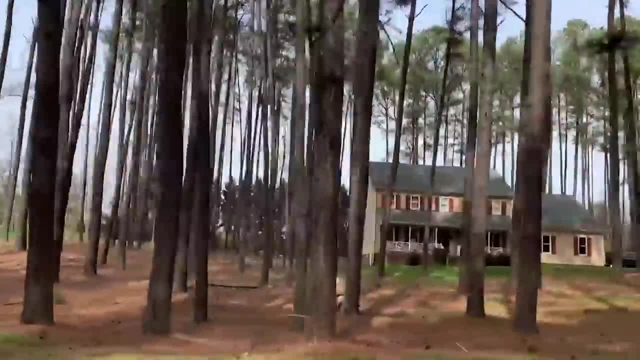 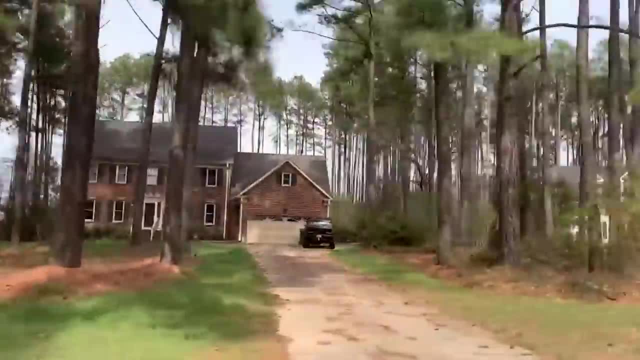 weekends here. It's growing super fast here in Cary because people all over the Midwest and Northeast and even the West Coast who want safety and good schools and property that'll go up in value. they've heard about Cary and they're like: I am moving there, But it's one of the 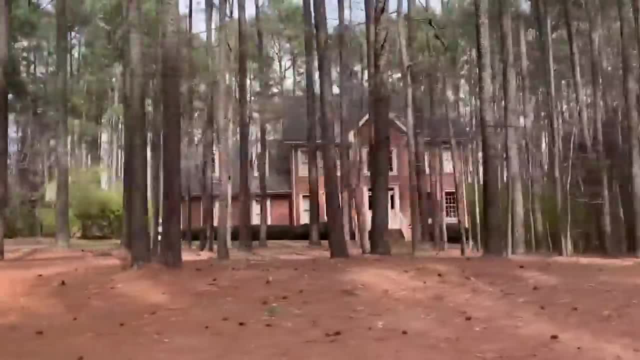 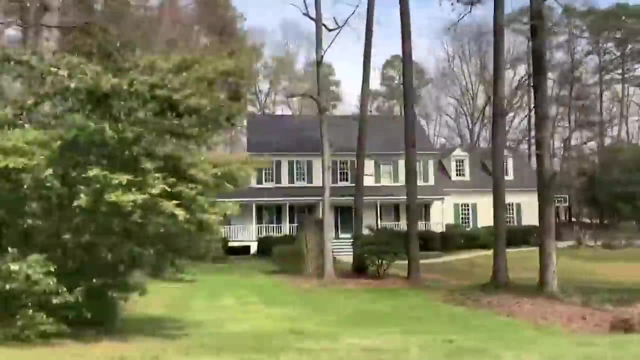 most expensive places in the state. It's one of the most expensive places in the state. It's one of the most expensive places to live too, because everyone's moving here. There just aren't enough homes. We're talking 400 to 500K, but Cary is the bee's knees. folks, There's tons. 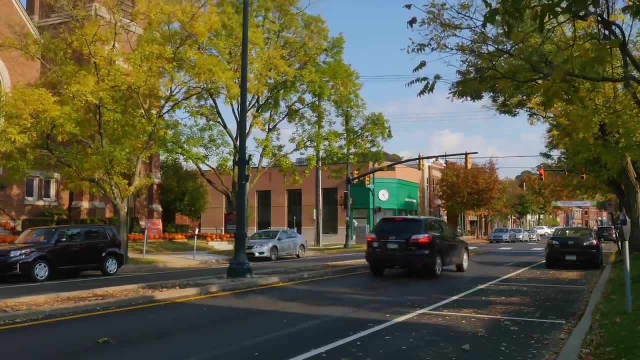 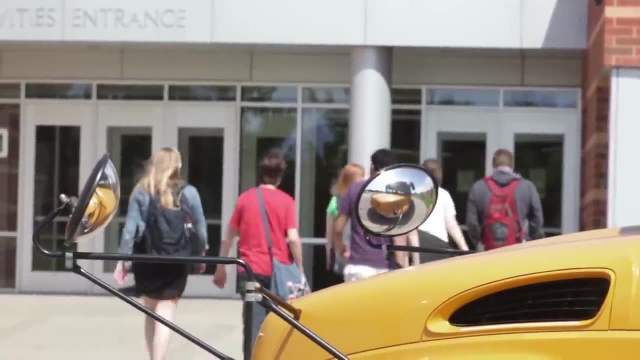 of parks. There's shopping around every corner. You don't even have to leave Cary. Everything's right in Cary's city limits. Schools are great. It's super clean. I mean it's almost too clean. Parts of Cary are so clean and modern. they look fake. People just take pride in living in Cary. I'll tell you that Where's the best place to live. What's better than Cary? It's actually Davidson, a suburb of Charlotte. Hey, for only the third time we're outside of the Raleigh metro area. Davidson's a little small college town that's growing really fast. It was 5,000 people here. 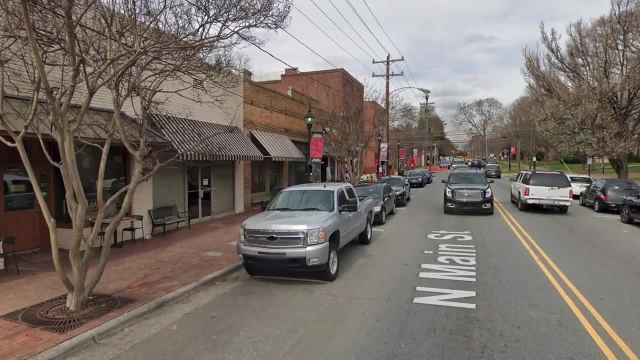 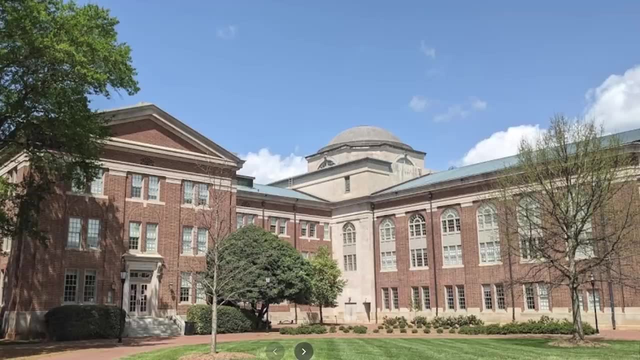 20 years ago. Now there's like 14,000 people. It's clear that people love living here, though, and they're proud of their town. Everybody here has a great job or they're retired. I mean the unemployment rate's lowest in the state. It's a college town, home to Davidson College. 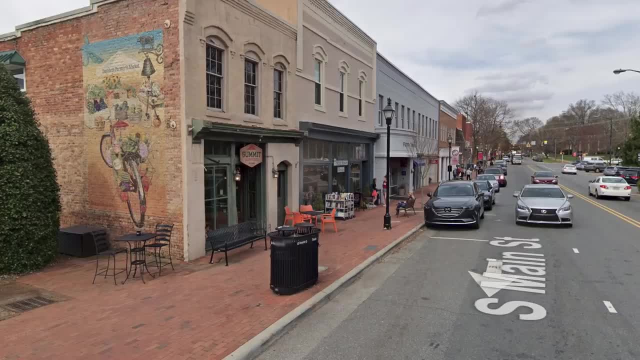 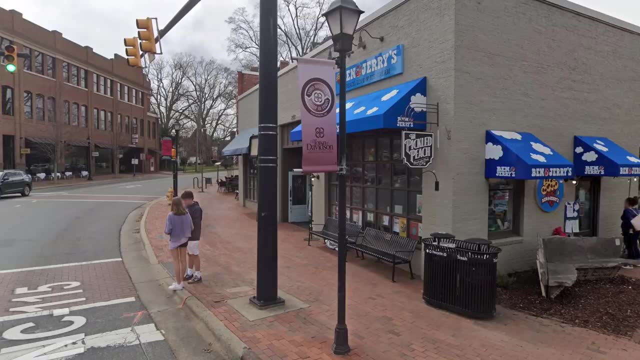 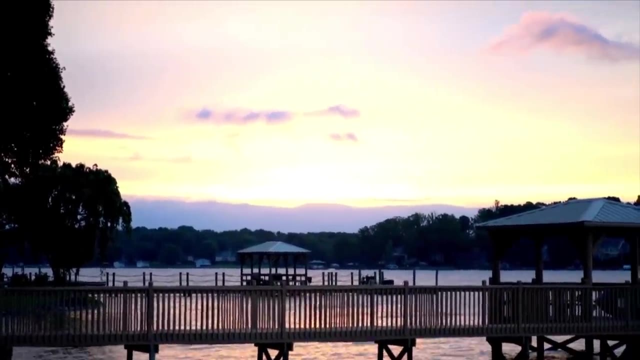 which is a really beautiful campus. It's a college town. Half the population has a college degree. There's cute shops everywhere and restaurants, and everybody here is really super friendly. And one of the best parts about living in Davidson Lake Norman. It's the largest man-made lake in the state, with over 520 miles of.